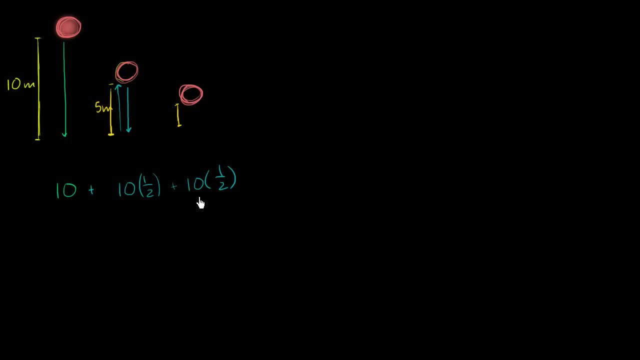 So it's going to go up 10 times 1 half, up 5 meters, And then it's going to go down 10 times 1 half. It's going to go down 5 meters. So it's going to travel a total vertical distance of 10 meters. 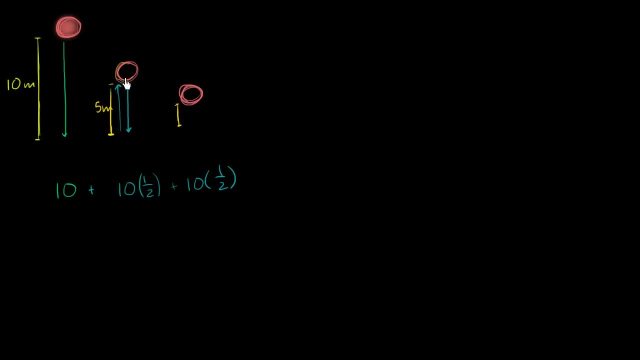 5 up and 5 down. Now, what about on this jump, or on this bounce? I should say, Well, here it's going to go half as far as it went there. So it's going to go 10 times 1, half squared up. 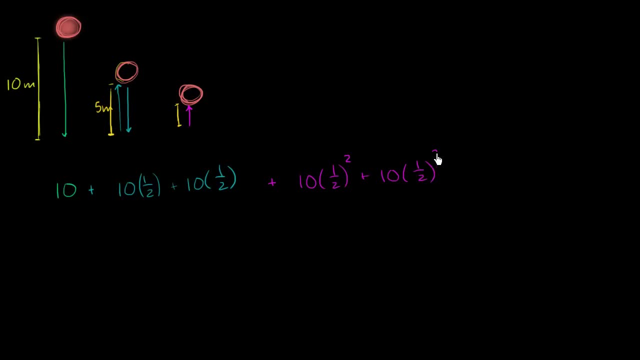 and then 10 times 1, half squared down, And I think you see a pattern here. This looks an awful lot like a geometric series, an infinite geometric series. It's going to just keep on going like that forever and ever, So let's try to clean this up a little bit. 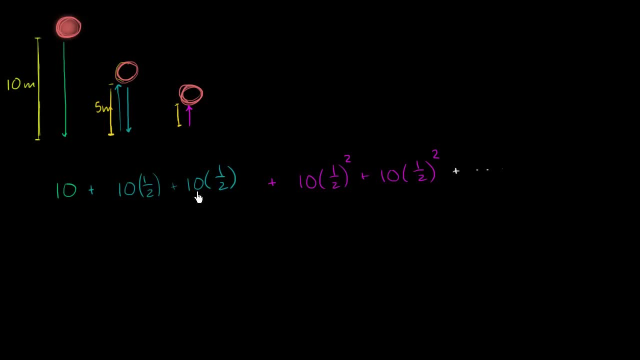 so it looks a little bit more like a traditional geometric series. So if we were to simplify this a little bit, we could rewrite this as 10 plus 20 times 1 half to the first power Plus 10 times 1 half squared plus 10 times 1 half squared. 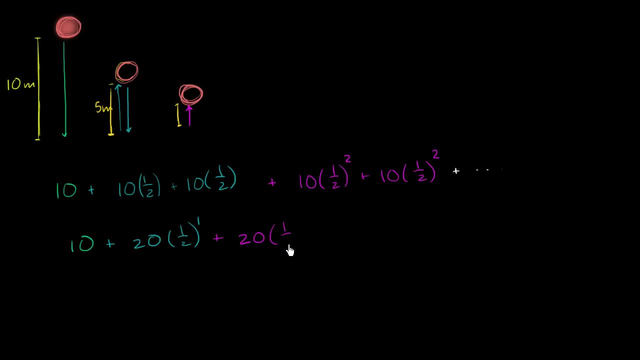 is going to be 20 times 1, half times 1, half squared, And we'll just keep on going on and on. So this would be a little bit clearer if this were a 20 right over here, But we could do that. 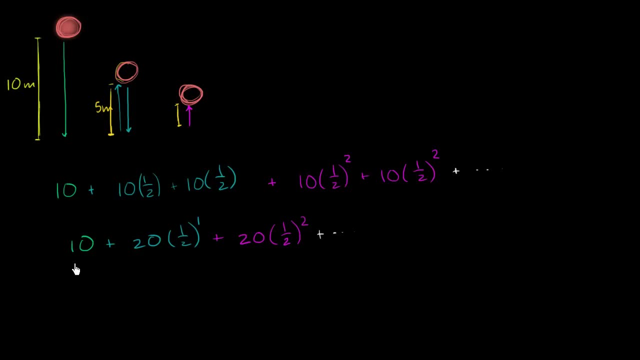 We could rewrite negative 10, or, sorry, we could write 10 as negative, 10 plus 20.. And then we have, plus all of this stuff right over here, Plus 10.. Plus all of this. Let me just copy and paste that. 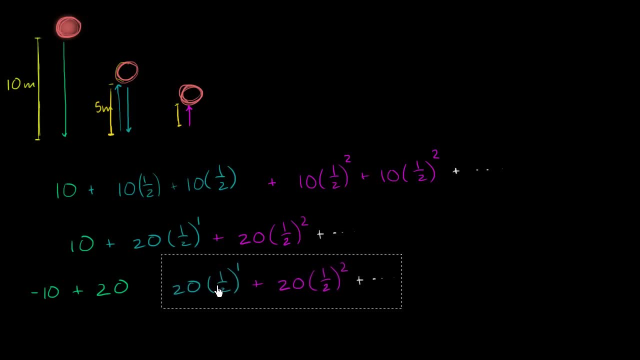 Copy and paste. So, plus all of this right over here, And we can even write this first, We can even write this 20 right over here. It's 20 times 1 half to the 0 power, 20 times 1 half to the 0 power. plus all of this. 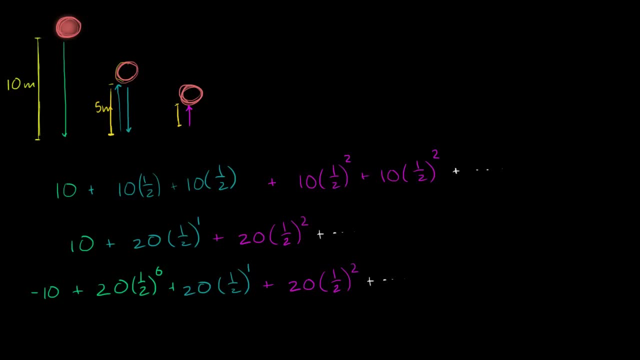 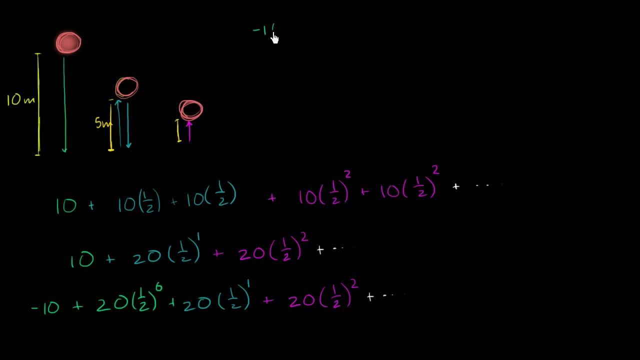 So now it very clearly looks like an infinite geometric series. We can write our entire sum And maybe I'll write it up here, since I don't want to lose the diagram. We could write it as negative 10.. That's that negative 10 right over here.